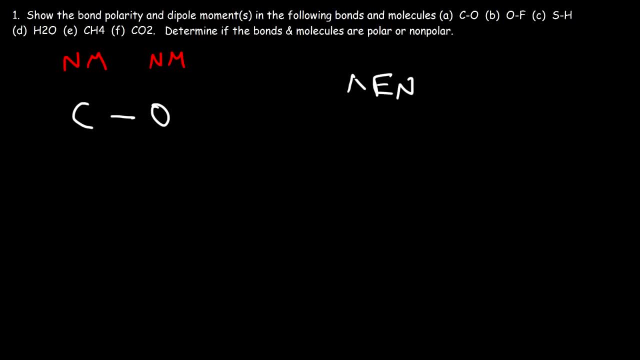 If the EN difference is less than 0.5,, then what you have is a nonpolar bond. If the electronegativity difference is greater than 0.5, then you have a polar covalent bond. Carbon has an electronegativity value of 2.5, and oxygen is 3.5. 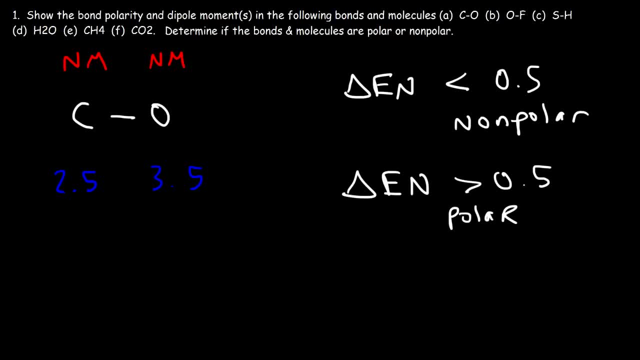 If you need access to these numbers, I suggest that you go to Google Images and type in electronegativity values from the periodic table or something like that. Now, going back to this, we can see that the The electronegativity difference in this molecule is 3.5 minus 2.5, so that's 1.0. 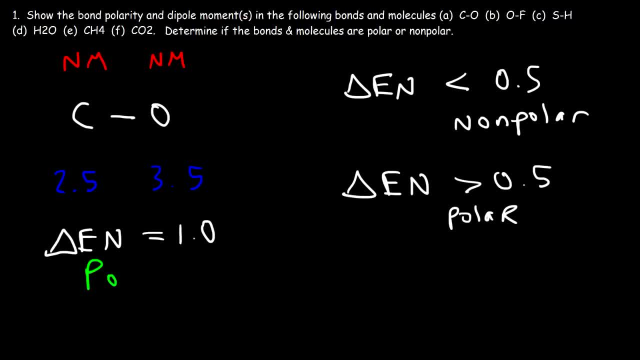 So, therefore, the carbon-oxygen bond is a polar bond or a polar covalent bond. Now that we know that oxygen is more electronegative than carbon, we can indicate the bond polarity: Oxygen has a partial negative charge and carbon has a partial negative charge. 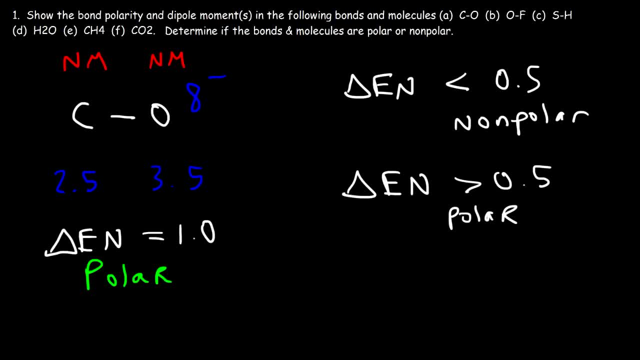 Oxygen has a partial positive charge. Now, to draw the dipole moment, you need to draw an arrow that starts from the positive part of the molecule and points towards the negative part of the molecule. So this is the dipole moment and this represents the bond polarity. 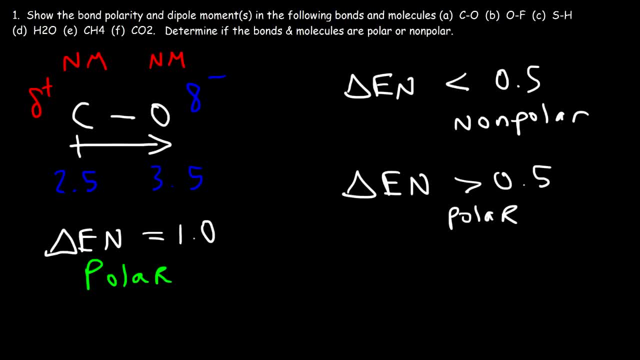 Now, whenever you have a net dipole moment, the molecule as a whole is polarized. If all the dipole moments cancel, then the molecule as a whole is nonpolar. But we'll talk about that later. Let's move on to our second example, the oxygen-fluorine bond. 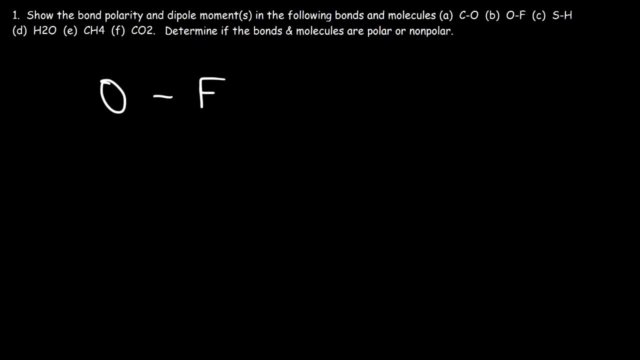 So go ahead and indicate the bond polarity and the dipole moments for this bond and determine if it's polar or nonpolar. So let's look at the EN values first. Oxygen has an electronegativity, The value is 3.5, and fluorine is 4.0.. 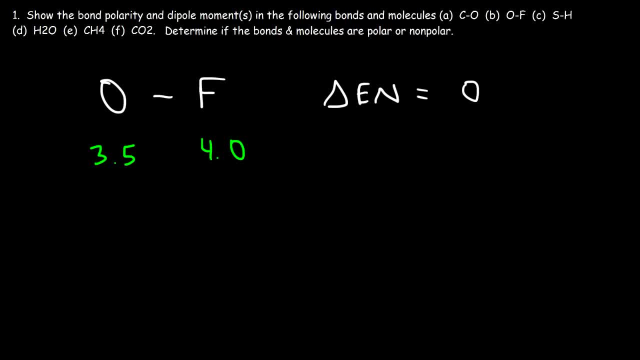 So the EN difference is 0.5, which makes this a polar covalent bond. Both oxygen and fluorine are nonmetals And whenever you have two nonmetals combined, typically they form covalent bonds. But we have a polar covalent bond because fluorine and oxygen- they don't share the electrons equally. 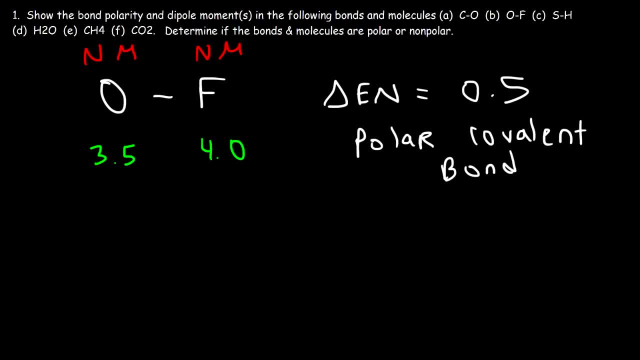 Fluorine is going to pull the electrons apart. Fluorine is going to pull the electrons apart. Fluorine is going to pull the electrons apart And, because it's more electronegative, it's going to acquire a partial negative charge. 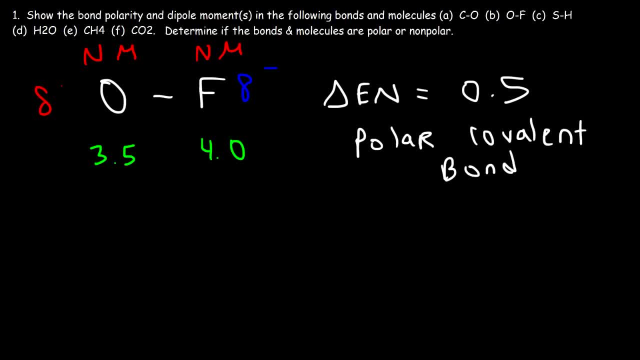 Whereas oxygen is going to be electron deficient. it's going to have a partial positive charge. So that's the bond polarity of the oxygen-fluorine bond. Now the last thing that we have to draw is the dipole moment And just point the arrow to the element that is most electronegative, in this case fluorine. 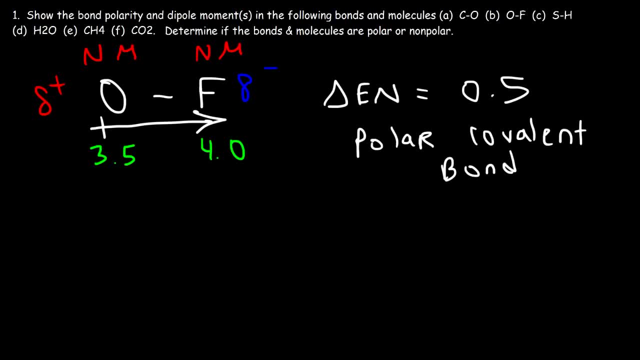 And so that's the dipole moment. That's the dipole moment of the OF bond. Now let's move on to part C, The sulfur-hydrogen bond. Sulfur is a nonmetal and hydrogen is a nonmetal. 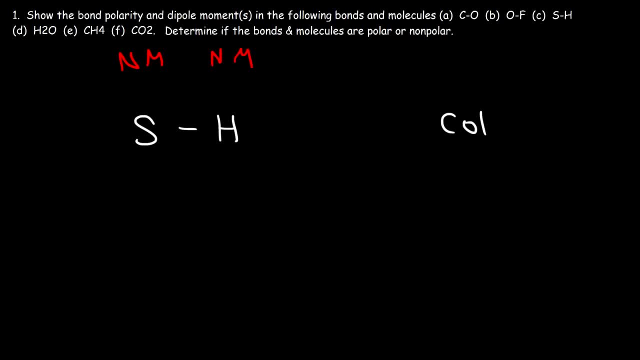 So, therefore, this is going to be a covalent bond. Now, is it going to be a polar covalent bond or a nonpolar covalent bond? By the way, if we had a metal and a nonmetal, typically it would represent an ionic bond. 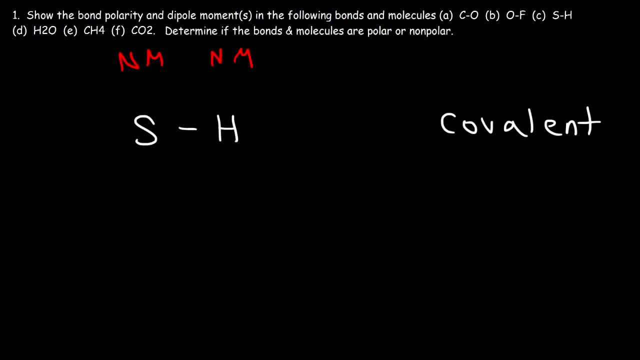 So this is going to be a nonpolar covalent bond. Hydrogen has an electronegativity value of 2.1. And sulfur that is about 2.5. And so the electronegativity difference is 0.4.. 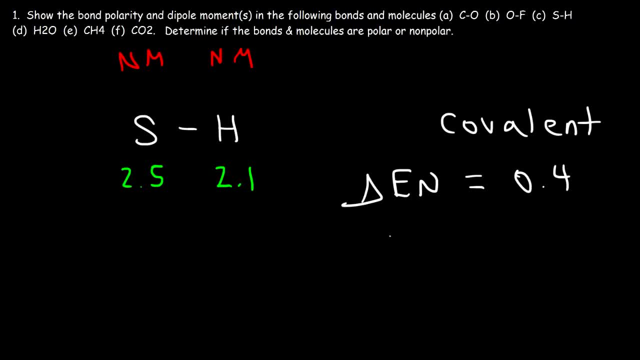 Which means that the hydrogen-sulfur bond is relatively nonpolar. So what we have is a nonpolar covalent bond, And so this is going to be a nonpolar covalent bond. Sulfur is more electronegative than hydrogen. 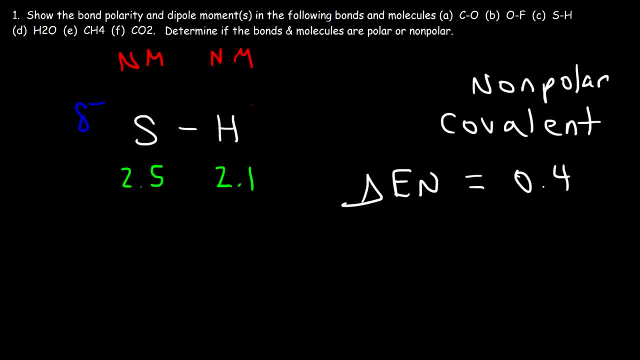 So sulfur is going to have the partial negative charge And hydrogen is going to bear the partial positive charge. So, to draw the dipole moment, we're going to point the arrow towards the more electronegative sulfur atom, And so that's it for that example. 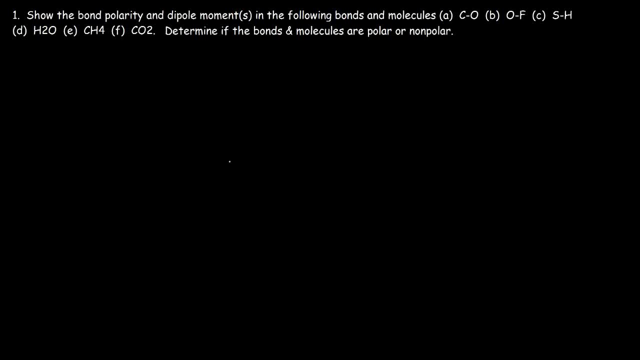 So now, what about molecules? So here's how you draw water. So that's a simple Lewis structure of the H2O molecule. So, given this molecule with the appropriate geometry, indicate the bond polarity and the dipole moment. So first let's focus on the oxygen-hydrogen bond. 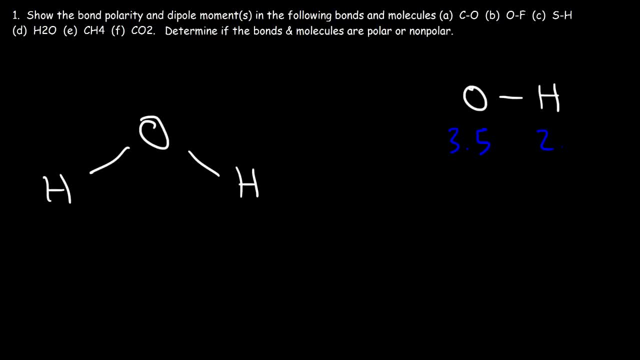 Oxygen is 3.5 and hydrogen has an EN value of 2.1.. So oxygen bears the partial negative charge and hydrogen bears the partial positive charge. So we're going to accumulate these fixed values. So this bond is a polar covalent bond. 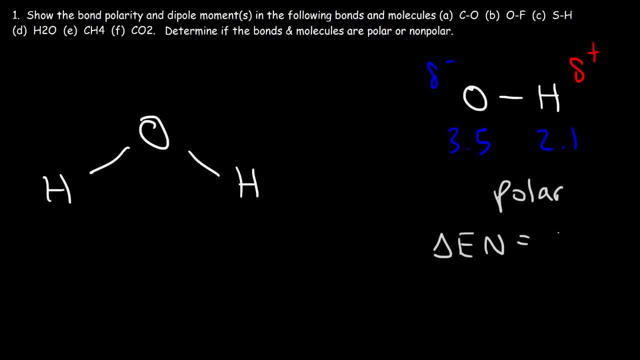 The electronegativity difference is 3.5 minus 2.1, and that's 1.4.. So it's much greater than 0.5.. And the dipole moment of this bond is going to point towards the oxygen atom. 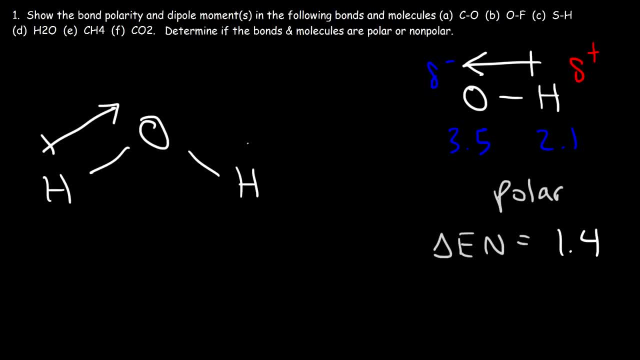 So the OH bond is polar. Now if we draw the dipole moments from the molecule- the bond polarity- we know that hydrogen is going to have a partial positive charge and there's two of them. so oxygen needs a partial negative charge. that's twice the value we got to put a 2 in front of it so it can neutralize these. 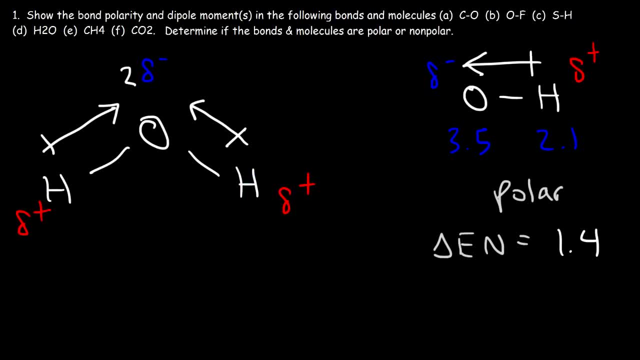 two partial positive charges. so make sure you put that 2 in front. and so that's how you can indicate the bond polarity and the dipole moment of a molecule. so now we need to ask the final question: is the molecule polar or nonpolar? because you can have a molecule with polar bonds, but overall the 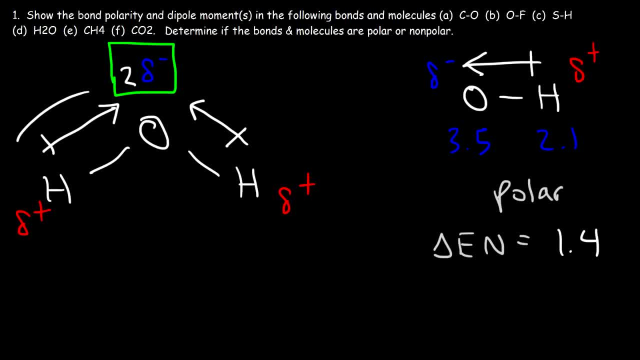 molecule itself may be nonpolar, and so you need to look at the arrows, the dipole moments. so we have one arrow going this way and the other arrow going this way. for the molecule as a whole to be polar, you need to have a net dipole moment. 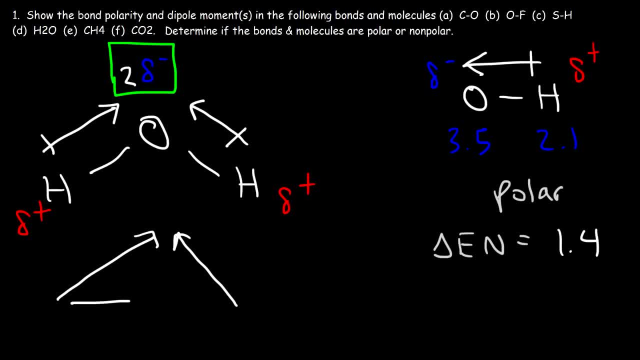 based on the way this molecule is drawn, notice that the X components of the arrows cancel, so these two opposite in direction to cancel. but the Y components do not cancel, they point in the same direction. so therefore this molecule has a net dipole moment in a positive Y direction. 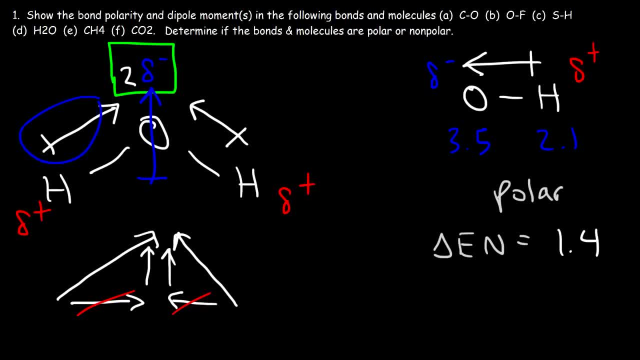 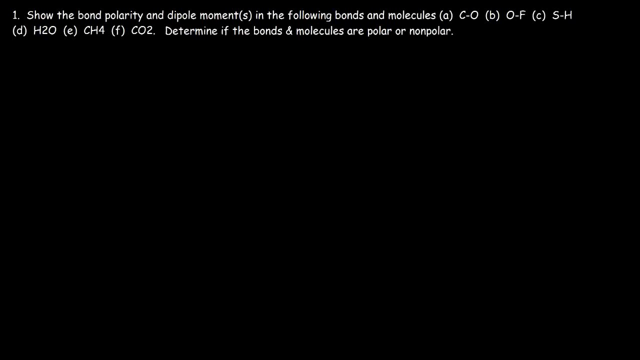 so because there's a net dipole moment and these two arrows do not completely cancel, we could say that the molecule as a whole is polar. now let's consider methane- CH4. methane has a tetrahedral structure, so it's not easy to represent it on this screen because it's a three-dimensional object. 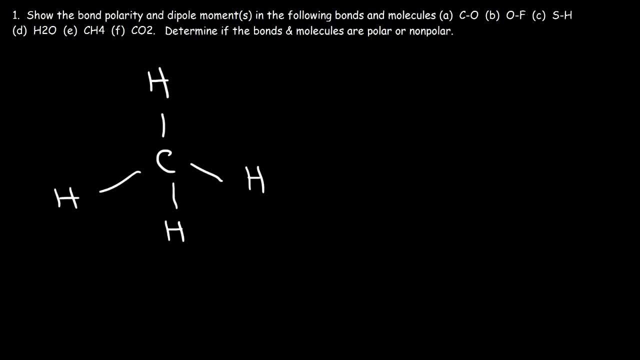 not a two-dimensional object. now, the carbon-hydrogen bond is nonpolar. the electronegativity difference is less than 0.5, fact it's .4. however, carbon stills bears the negative charge and hydrogen bears the partial positive charge. so to indicate the bond polarity of methane, we 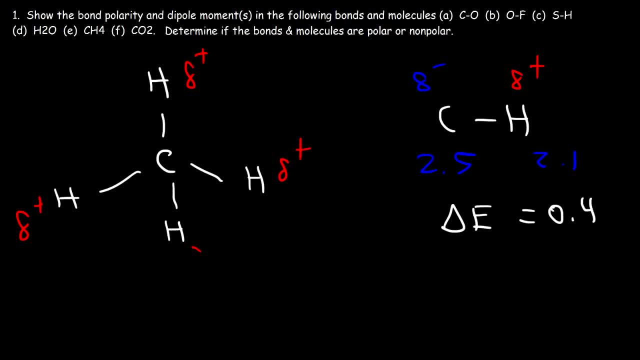 need to show the four partial positive charge of every hydrogen atom. for carbon it's gonna have a negative charge, but we're gonna multiply by 4 due to these four charges. so that's the bond polarity of the molecule. now the dipole moment is going to be negative. 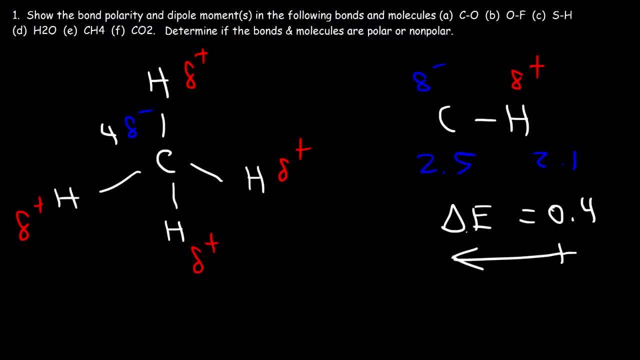 to point towards the electronegative carbon atom. So we have one going here, another going there. and if you draw this molecule, its 3D structure, and you look at the arrows correctly, or if you really analyze it the way, this structure 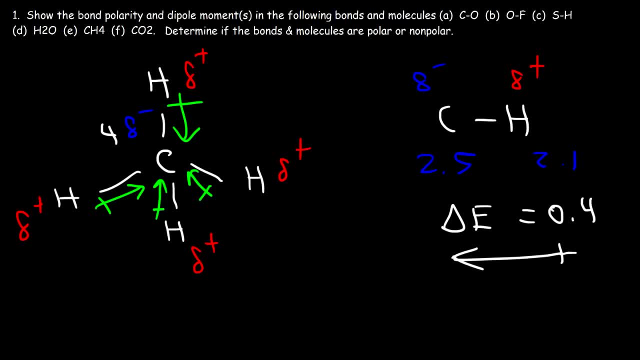 is set up. it's set up in such a way that all of the dipole moments completely cancel each other, so that the net dipole moment is zero. So what we have is a molecule that contains non-polar bonds and, at the same time, the 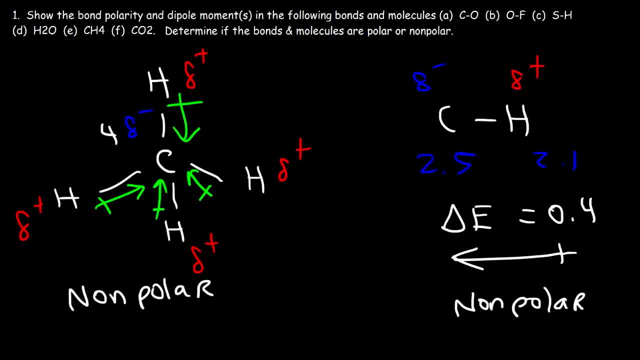 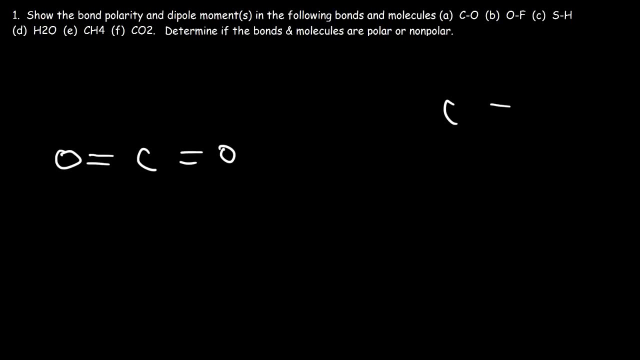 molecule as a whole is non-polar overall. Now let's look at our last example: carbon dioxide. So I'm going to give you the Lewis structure of this molecule. it looks like this, So go ahead and work on that problem. The electronegativity difference between these two atoms is 1.0.. 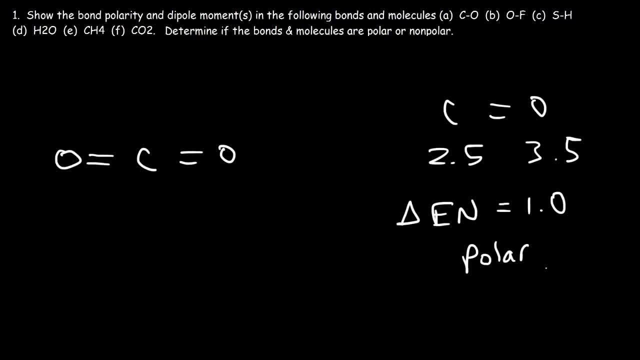 So what we have is a polar covalent bond. Carbon is partially positive with respect to oxygen, because oxygen is more electronegative than carbon, And so the dipole moment is going to point towards the electronegative oxygen atom.